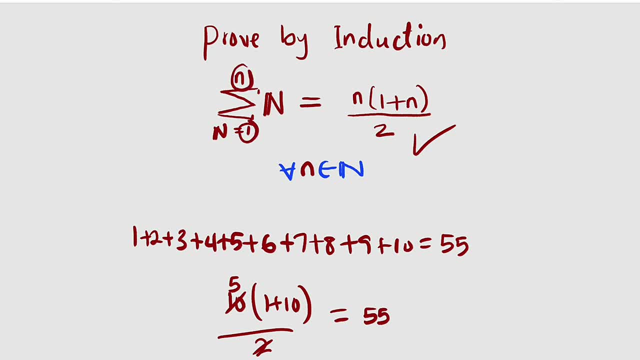 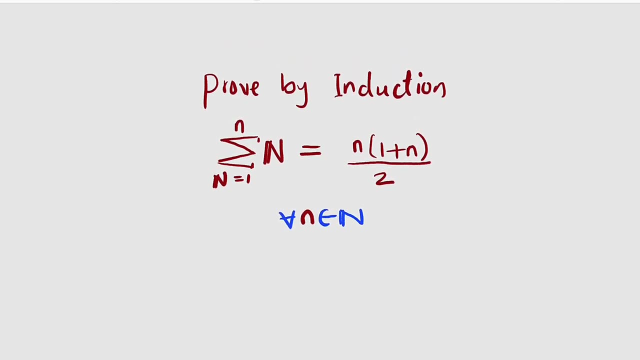 terms starting from 1 and you stop at n. So if you have n equal to 10, it will be equivalent to what we have just done here. Okay, let's get started with the solution. As you know, we have three basic steps. The step one: we are going to test for n equal. 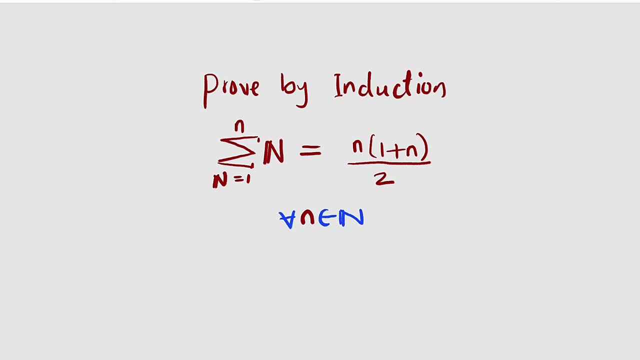 to 1, where 1 is the first term in the set of natural numbers. So we say Step 1.. All we have to do is to substitute the value of n equal to 1.. So it means that from the left hand side we are going to begin with 1 and stop at 1 meaning 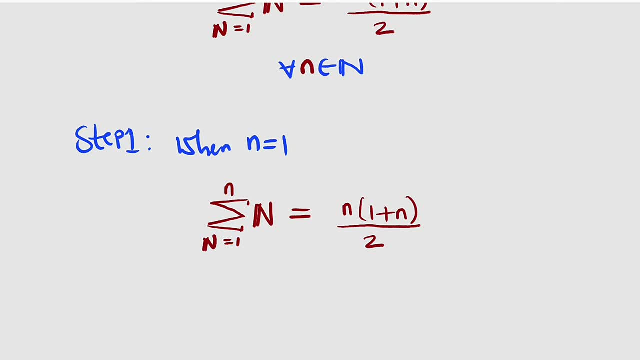 we have only a single term, which is 1.. The left hand side will be just 1.. Is the same thing as the right hand side. The right hand side will be 1 multiplied by 1 plus n is also 1 divided by 2. in the bracket we have 1 plus 1, which is 2, and 2 multiplied by the 1. outside is: 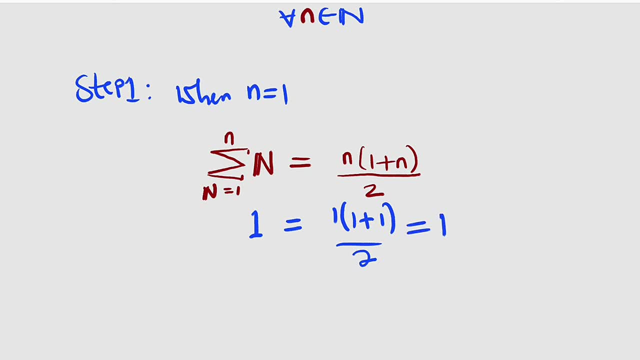 still 2. 2 divided by 2 is 1. so the right and the left hand side are all equal to 1. so in step 2 we want to assume a certain number in the set of natural numbers will also satisfy this statement if, and only if, 1 satisfied. so let us check another number in the set of natural numbers. 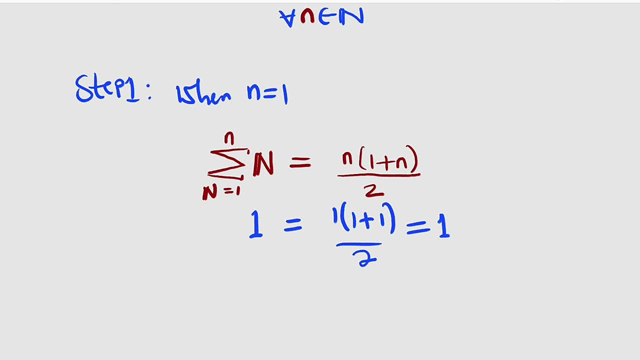 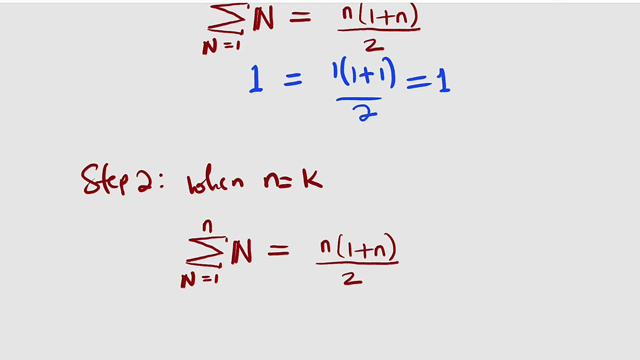 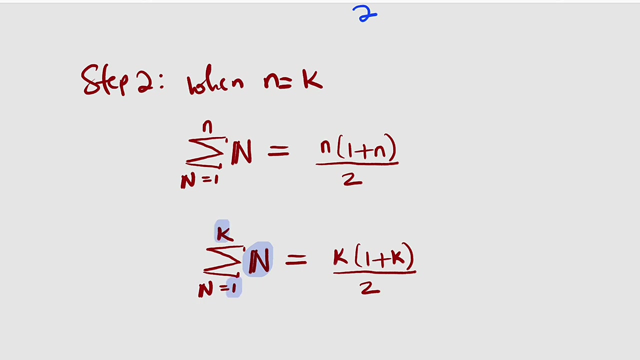 to see whether this is true. we are not going to use a number, rather a variable, for instance k. so in step 2 we are going to set n equal to k, for which k belongs to the set of natural numbers. so let me substitute: this will be summation of natural numbers from 1 to k. 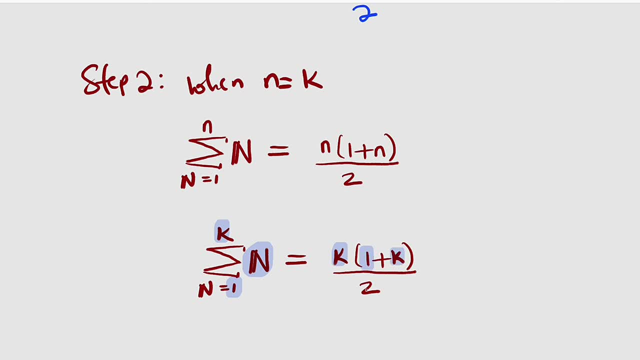 which is the same thing as k multiplied by 1 plus k divided by 2. so we are assuming that this is true, right? we just assume. we assume that this is true. if it is true, we are going to prove that any number after k will also satisfy this statement. for instance: 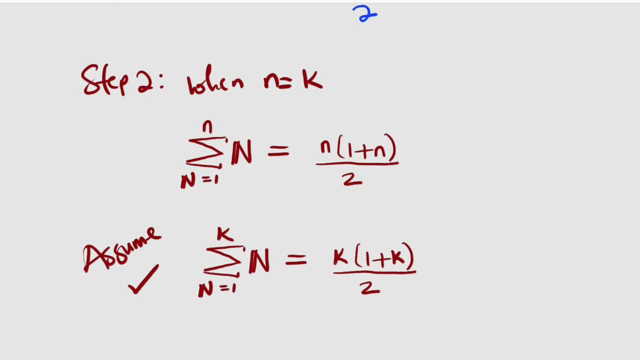 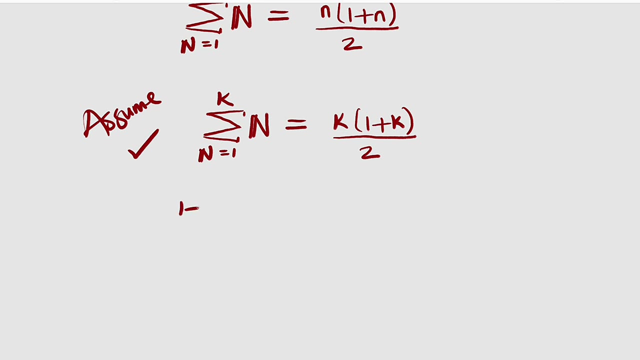 if seven satisfied the problem, we want to show that eight will also satisfy the problem, meaning seven plus one, which is the next time. so if k satisfied, we want to show that also k plus one will satisfy the problem. you know, the left hand side of this expression means 1 plus 2 plus. 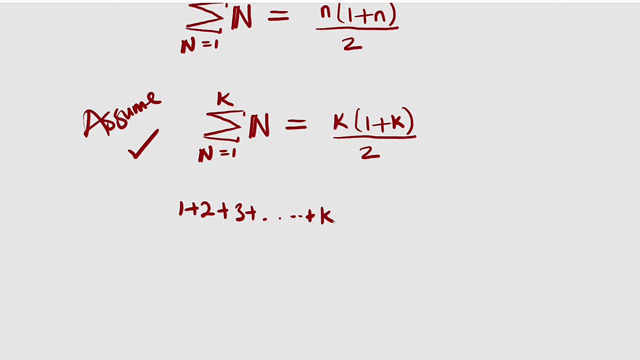 3 plus dot, dot, dot plus k. you know? this is exactly what it means. and the right hand side is k multiplied by 1 plus k divided by 2.. so if this is true, we want to prove that k plus 1 is also true. 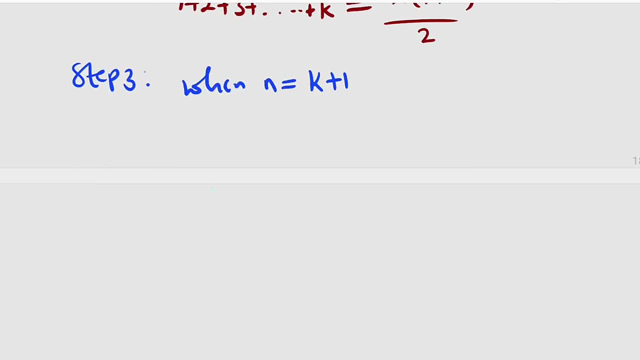 when n is equal to k plus 1.. this is what we have initially, so we are going to substitute n equal to k plus 1, since we have seen that k is true. so we have summation of n from 1 to k plus 1. 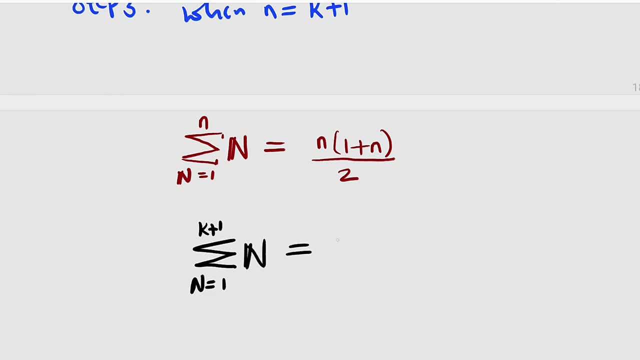 of these natural numbers equal to wherever we have n, we replace it with k plus 1. this is k plus 1 multiplied by. you know this is going to be k plus 1 plus 1. that will give us k plus 2, right k plus 2 divided by 2.. but remember the left hand side. it means we should be adding these numbers. 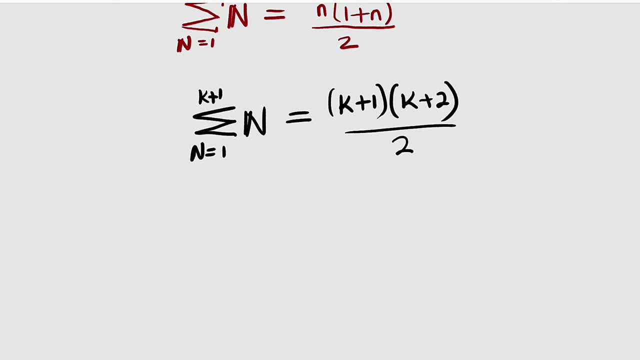 from 1 down to k plus 1, right? so let me break it down. this is the same thing as 1 plus 2 plus 3 plus dot dot dot plus k. you know, k is the number before k plus 1 plus k plus 1, right? this is the same thing as. 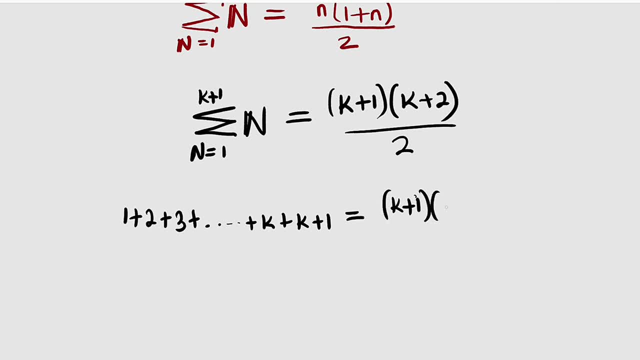 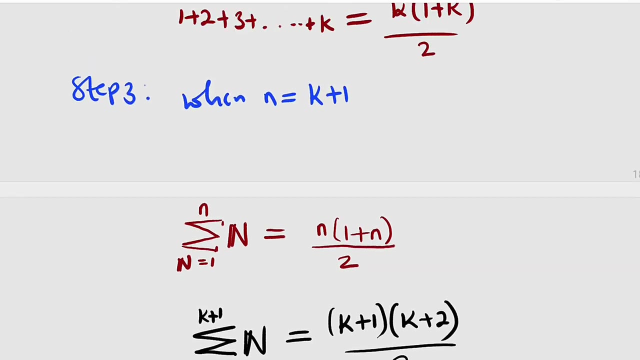 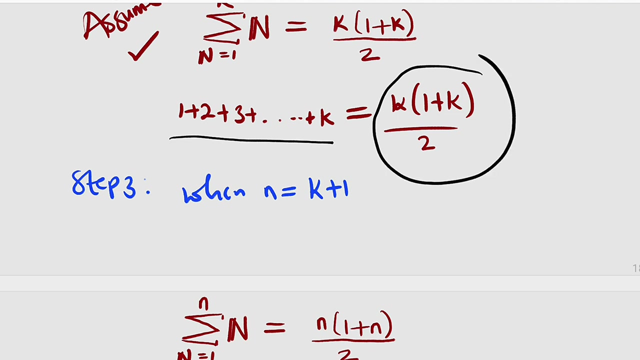 k plus 1 multiplied by k plus 2 divided by 2.. you should observe that from 1, 2 to k is familiar, right, because that's what we have to the right hand side from here. can you see that from 1 to k is exactly equal to this? therefore, we can substitute. 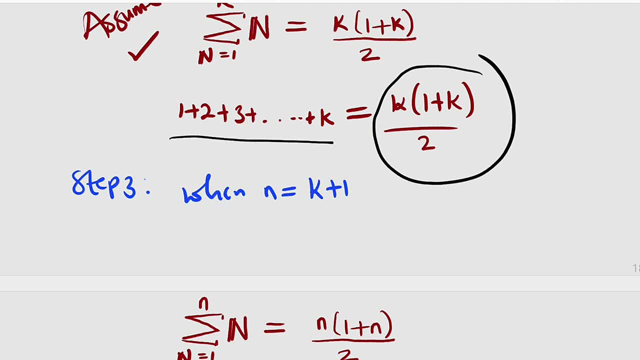 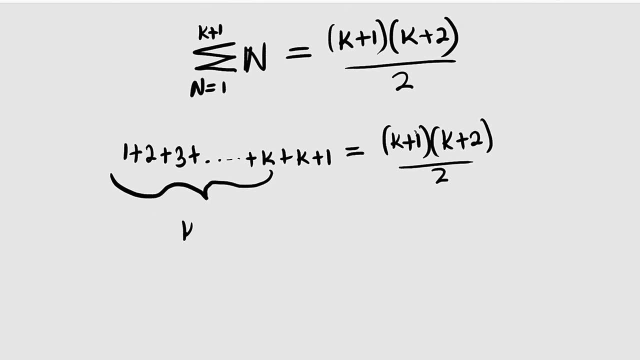 1 plus 2 plus 3 after k, with k multiplied by 1 plus k divided by 2.. so what we have here is just k multiplied by 1 plus k divided by 2, but we still have another k plus 1, right, we want to show that it is the same thing. 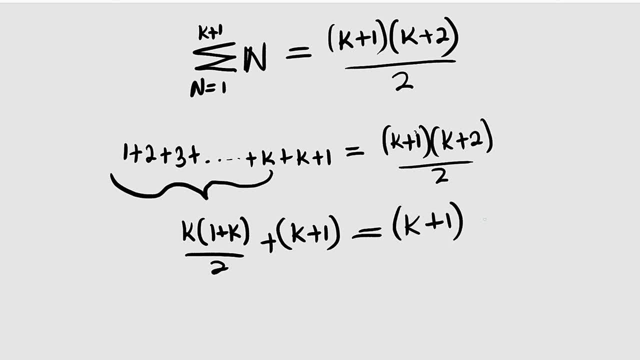 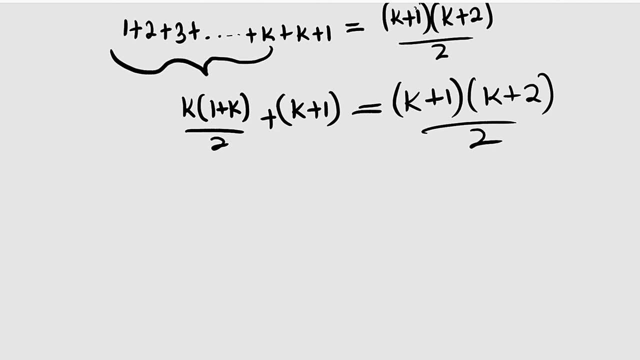 as the right hand side, which is k plus 1 multiplied by k plus 2, all divided by 2.. so let me just go ahead and simplify the left hand side, because we have already seen what the right hand side is. so we can rationalize this as divided by 1.. to make the denominators the 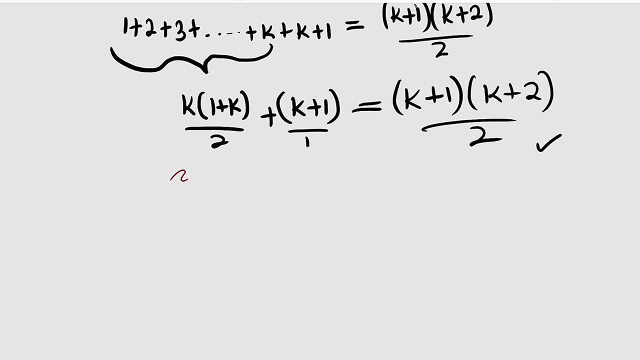 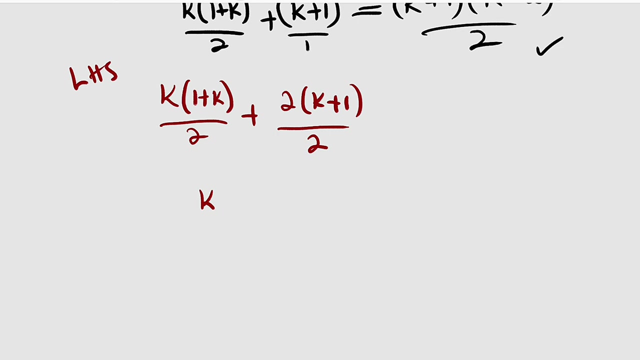 same. we can multiply the top and the bottom by 2, right. so we have k multiplied by 1 plus k divided by 2. then plus 2 of k plus 1 divided by 2. remember this is the left hand side. since we have common denominators, we can add denominators. this is k multiplied by 1 plus k. 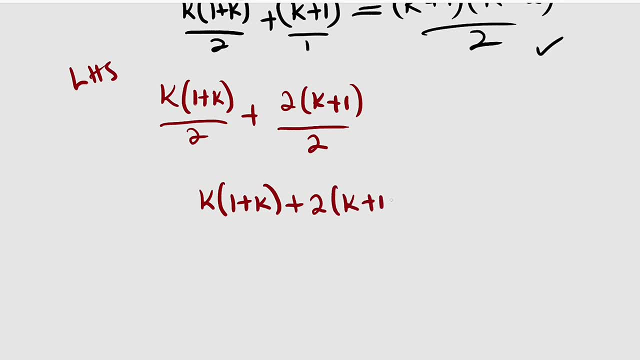 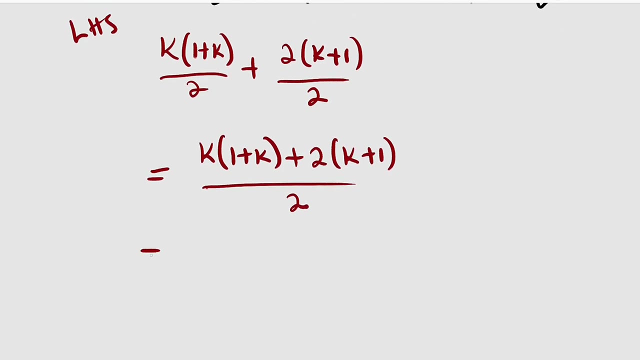 then plus 2, multiplied by k plus 1, the whole of this divided by 2, we take a common denominator. this can be factorized because you can see k plus 1 in common between the two times. so we factorize it as 1 plus k. if we factor 1 plus k outside, then inside from the first time. 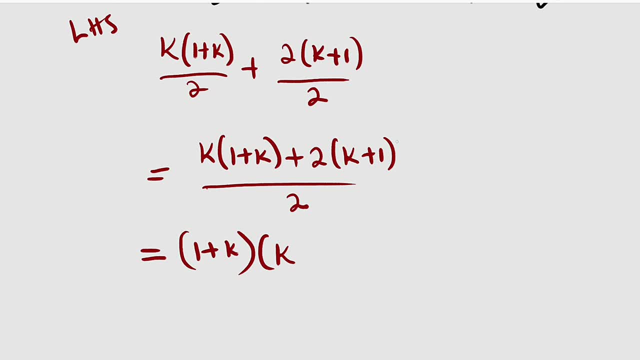 since this is gone, we have only k left from the second time. 1 plus k is gone. we have 2 left right. the whole of this divided by 2. remember, this is the left hand side, but observe that it is exactly the same thing we have done before. 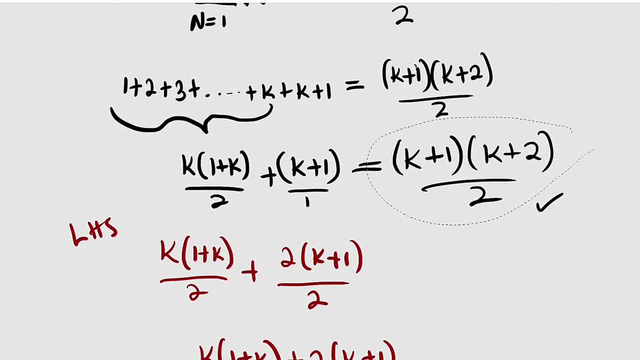 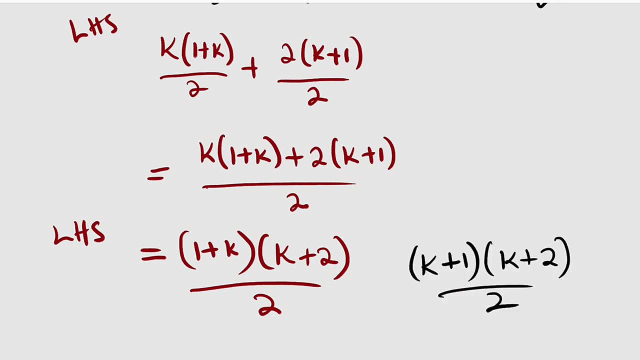 is exactly the same thing as the right hand side. let me just copy that: it is exactly equal to the right hand side. this is our right hand side and we want to always show that. whatever value you plug into this statement, the left and the right hand side will remain the same. and since the left and the right hand 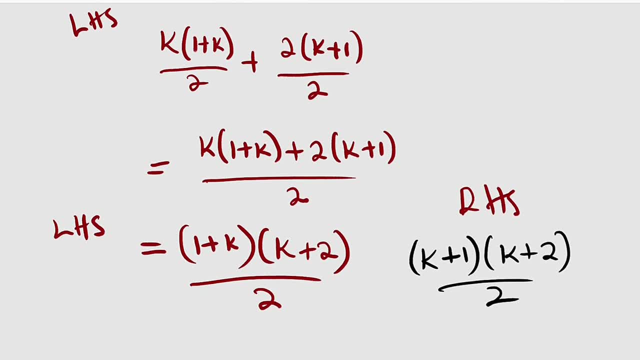 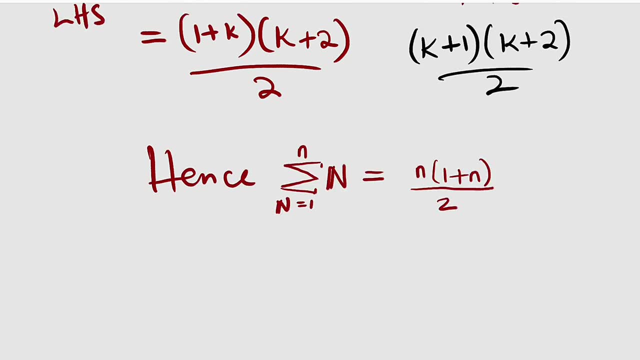 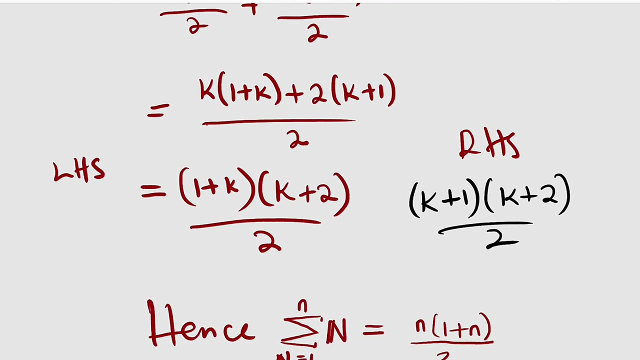 side are equivalent, then we conclude that this mathematical statement is true and hence this formula here is true for all n in the set of natural numbers. and this is all I have for you today. thank you for watching. do share to your learning colleagues and don't forget to subscribe to my youtube channel for more. 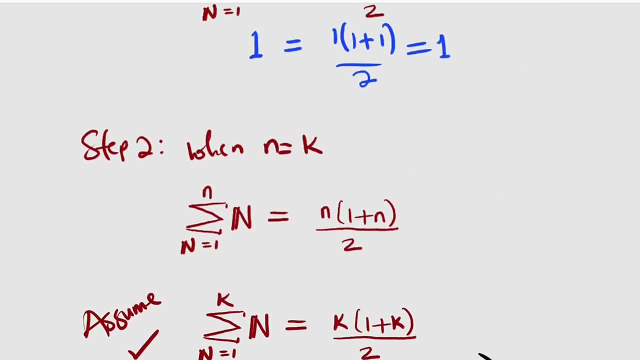 exciting videos, bye, bye.